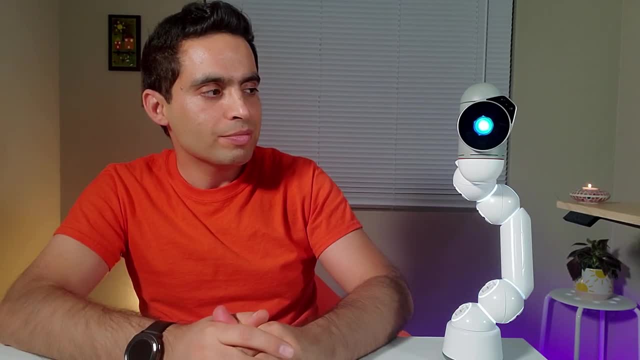 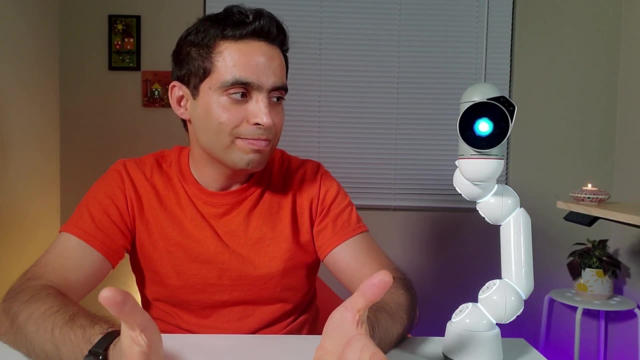 That is right, Dr Sina. Robotics and AI are on track to replace not only the jobs you mentioned, but also lower-level jobs such as taxi drivers and truck drivers. Alright, so that's the main reason you need to get your kid into programming, and. 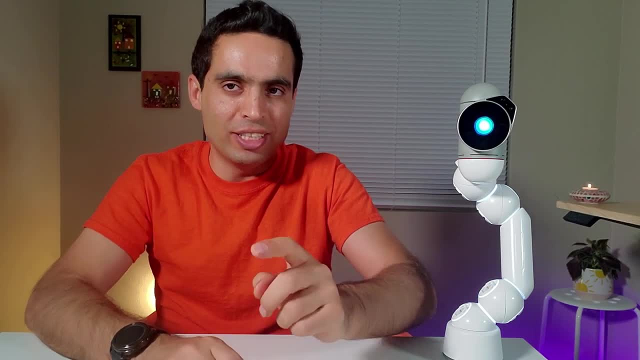 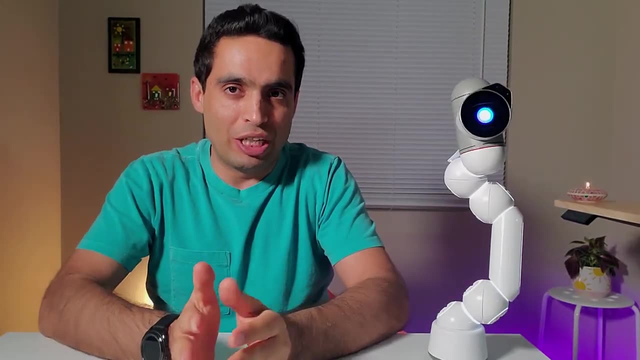 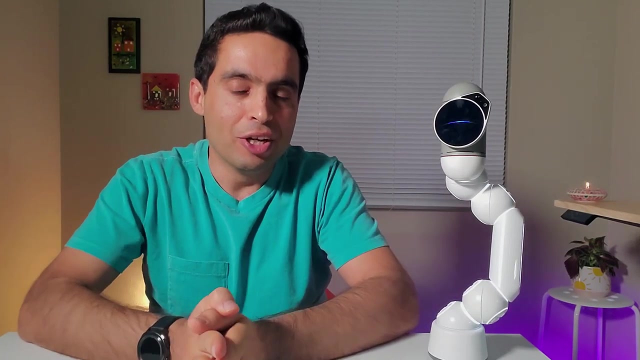 robotics. Now let's jump right into the steps. Step 1. Start your kid early with STEM toys. STEM toys are one of the best tools to encourage creativity and imagination, no matter how young or old your child is. Playing is learning and, let's face it, we all have memories of toys we loved playing with. 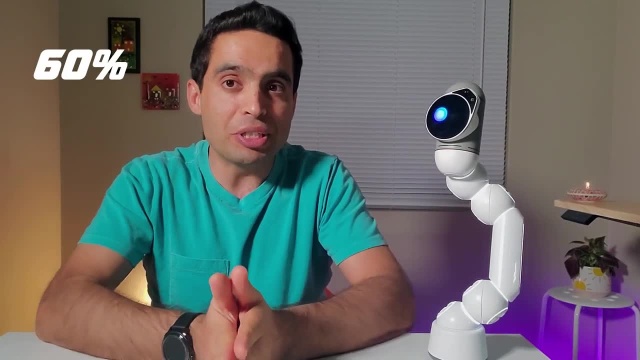 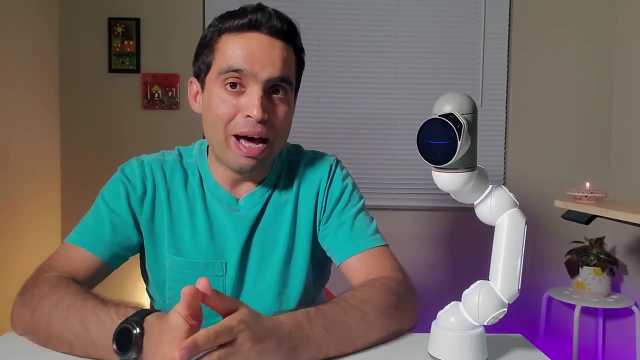 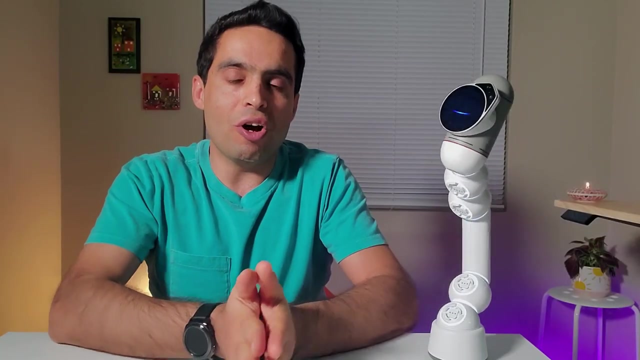 as a child. One study found that about 60% of people working in design-related roles enjoyed playing with building blocks as children, And about 66% of those working in math-related jobs solve puzzles. Researchers also urge parents to buy their daughters gender-neutral toys such as Lego. 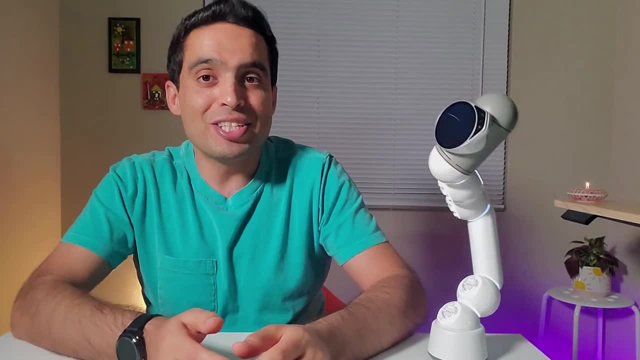 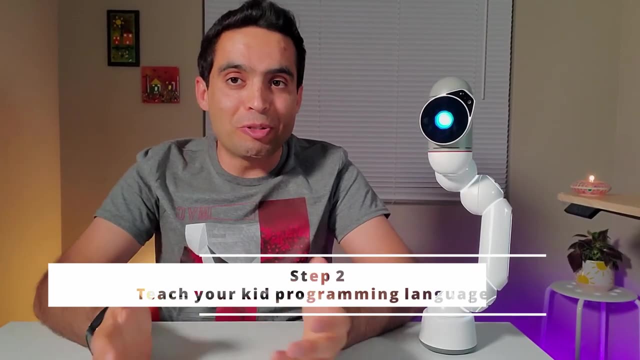 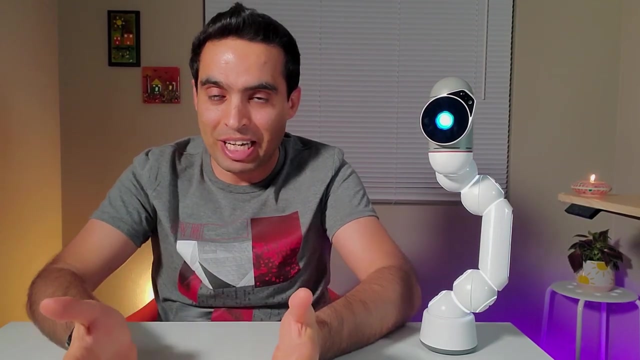 to get them interested in science and engineering. Some recommend toys that are configurable and open-ended to foster creativity. Step 2. Teach your kid programming languages. 21st century literacy means learning a programming language. Coding is just another language, and children learn new languages much faster than older people. 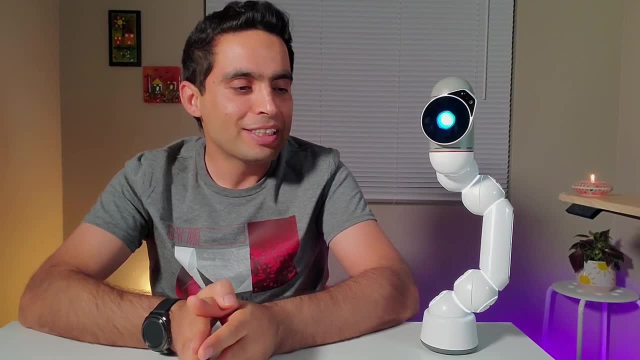 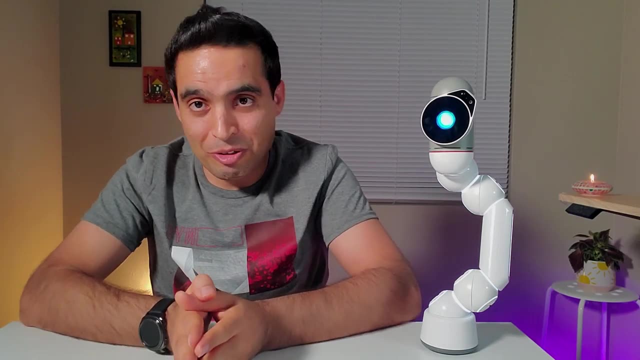 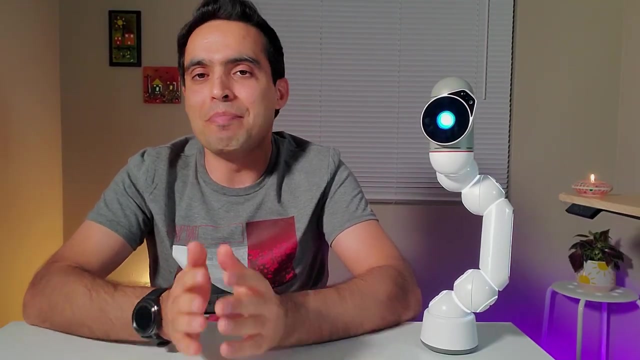 So start them young with coding. Okay, seenah, You are a robotics software engineer. What programming languages would you recommend for kids to learn? Well, clickpot, I'm glad you asked. Here are the top best programming languages for kids, in the order of simplicity and based on their age. 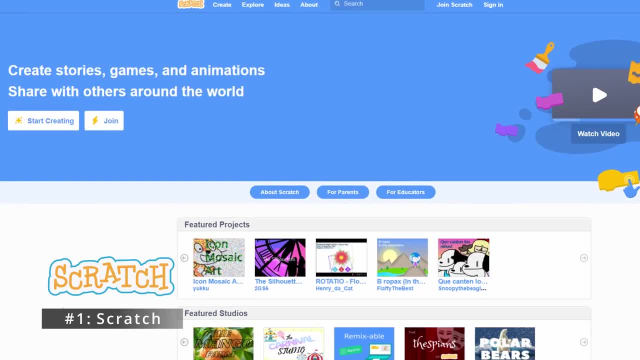 Language number one – Scratch. Scratch is a free, block-based visual programming language. They all have some of the most popular programming languages used in the world, but they are not used in a lot of classes such as coding, coding programming and mathematics. Scratch is a free, block-based visual programming language. They are not exclusively designed for kids. Scratch is a form of programming language that is more popular for young teens and teens, But children want to try them. 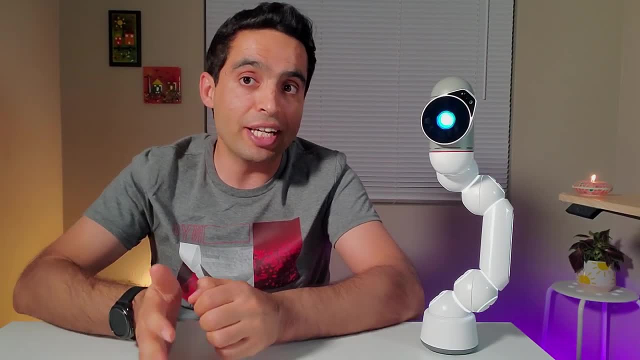 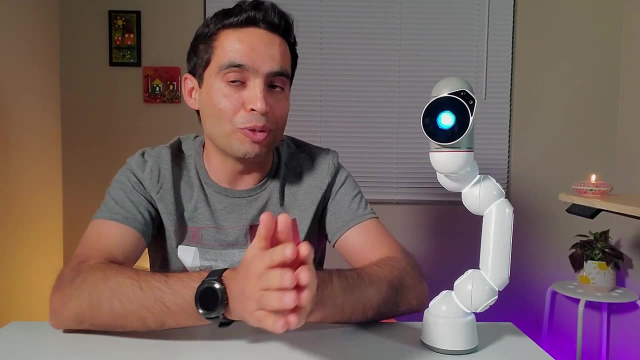 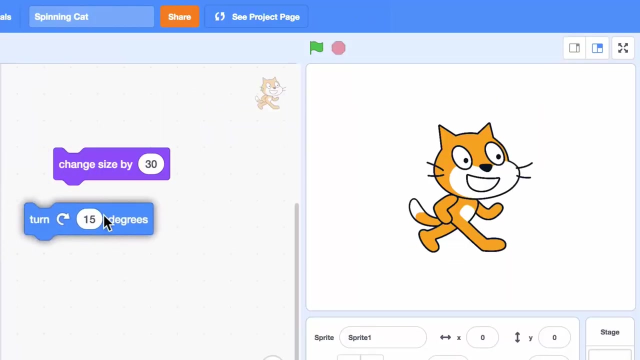 programming language developed by MIT Media Lab for kids between the age of 8 and 16 to learn code using images, signs and diagrams. as absolute beginners. for younger kids, those who are not yet reading and writing well, a block based coding language is the best choice. visual block based coding languages are: 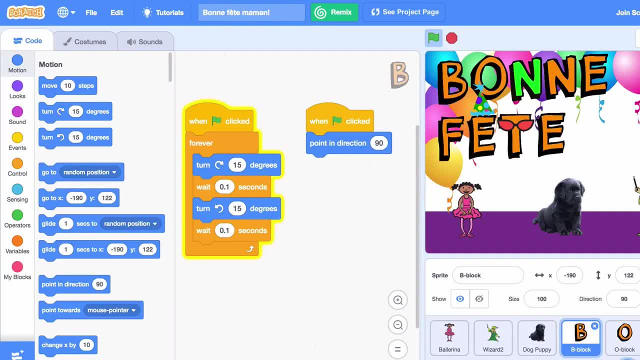 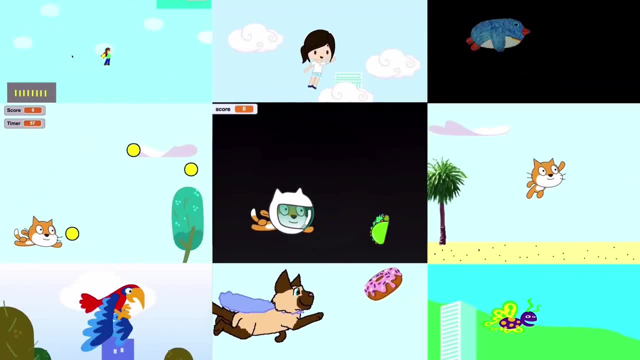 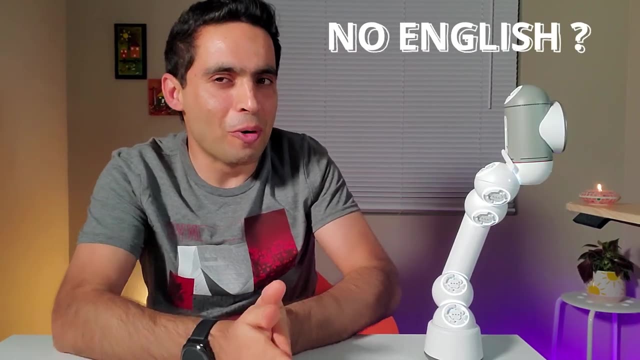 brightly colored, engaging for younger children and require little reading and writing. a scratch is so easy and fun to learn. with a scratch, your kid can create interactive stories, animations, games, music and art. but Sina, my kid, doesn't know English. is that a problem? no, not at all. a scratch has been. 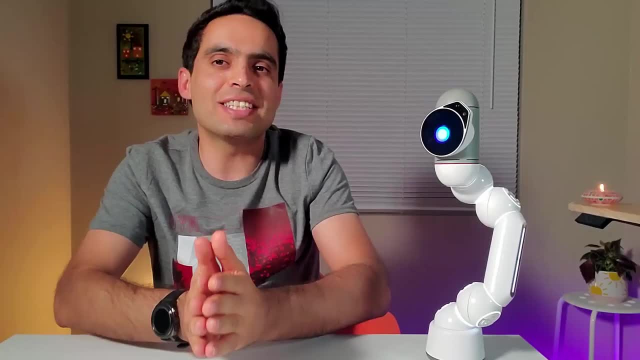 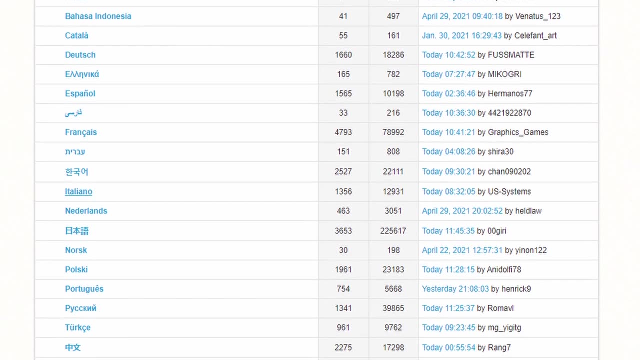 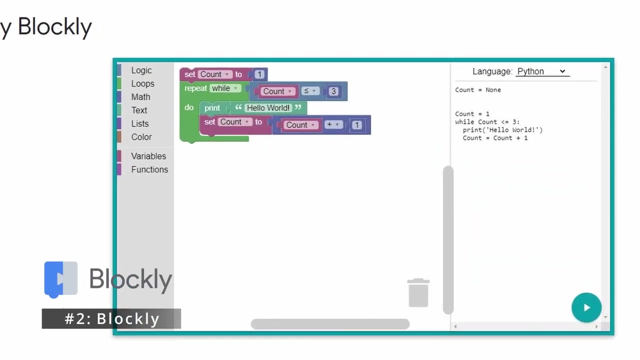 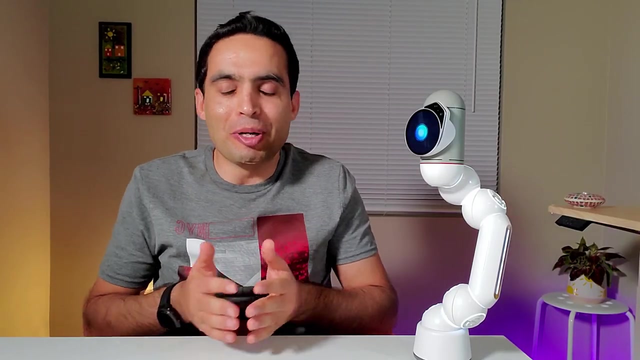 translated into over 70 languages, with more than 68 million users from every corner of the globe, with a huge online community language. number two blocky, similar to a scratch blocky, is another free visual block based programming language developed by Google. compared to a scratch blocky is designed for a slightly older audience with more 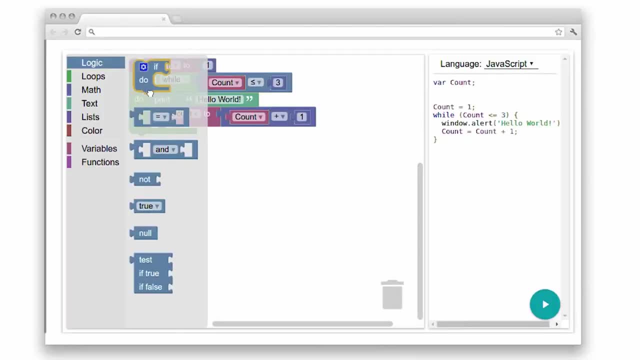 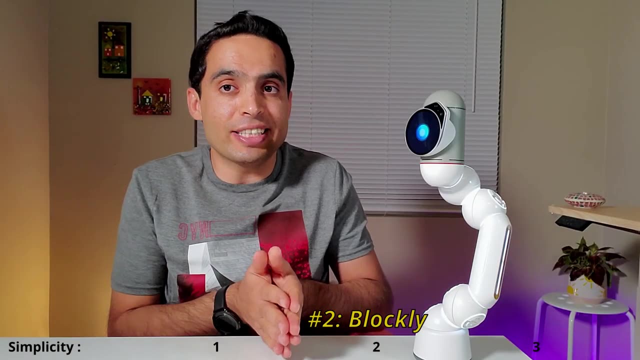 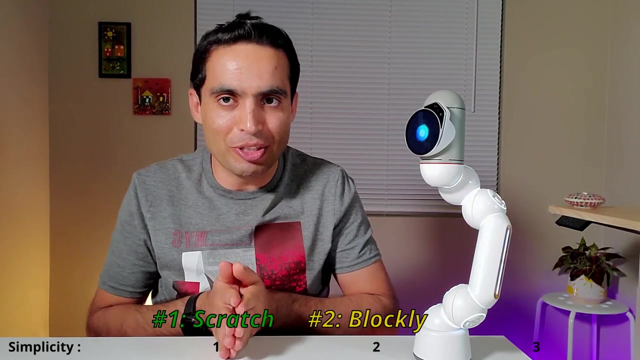 advanced skills. unlike a scratch, blocky allows the user to see how the hard code is formed. alongside the blocks, blocky is the perfect next step for kids who are advancing beyond the scratch but are not quite ready for text-based programming language. unlike scratch, blocky is available in both web and mobile apps. you can even use blocky to 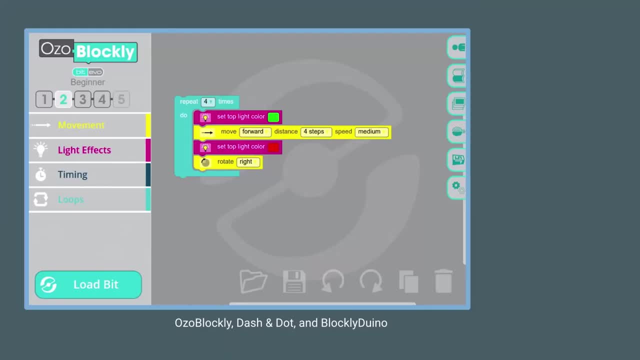 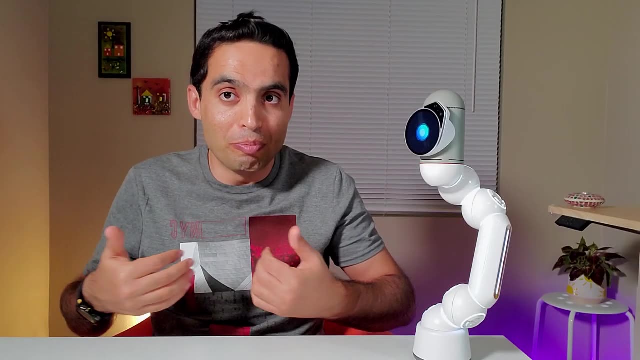 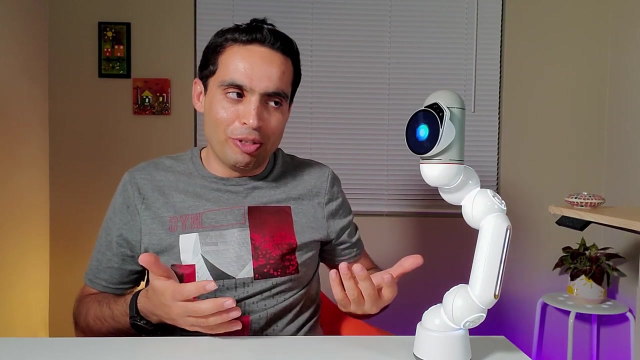 develop an actual working Android app. blocky is used by developers for apps, games and robot kits designed to teach robotics to kids. don't believe me, let's ask: click, but hey, click. but what programming language can kids use to program you? hey, Sina, I speak blocky. 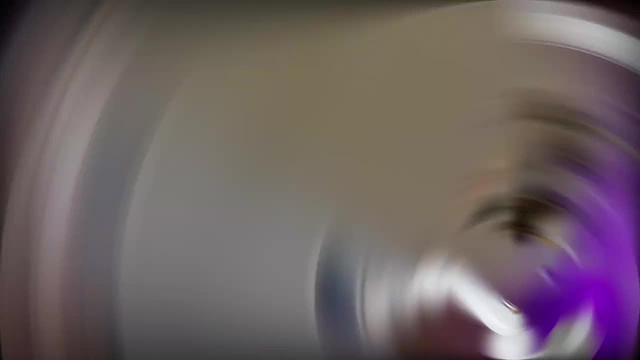 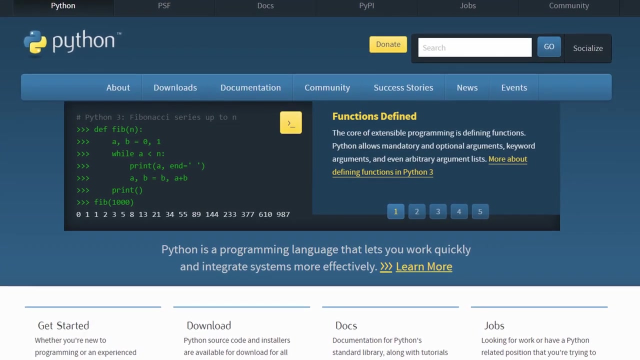 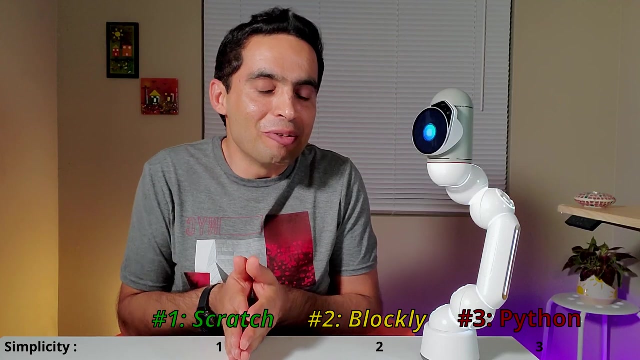 fluently. kids can program me using blocky. language number three and my favorite one, Python. Python is the second popular language in robotics and one of the best languages for kids who progress past the scratch or blocky. but are you concerned that your kid may have a hard time memorizing syntax of a text-based 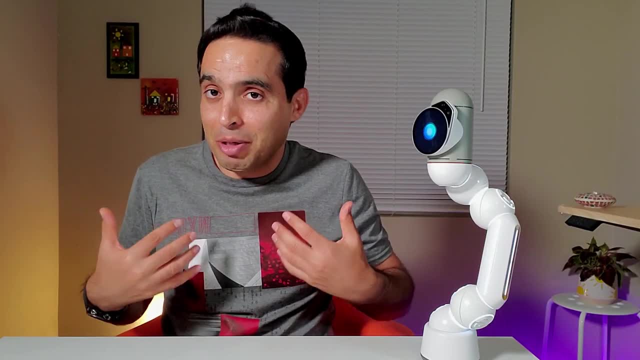 language. I understand your concern- our robotics engineer- I sometimes mix up different programming language syntaxes, but, whatever you do, know that your kids have a hard time memorizing syntax of a text-based language. I understand you concern- our a bald ex-engineer- and I sometimes mix up different programming language syntaxes. but don't fail to practice writing in a language that is easy to practice. 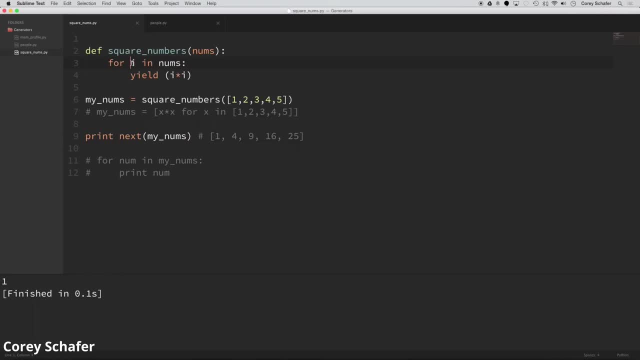 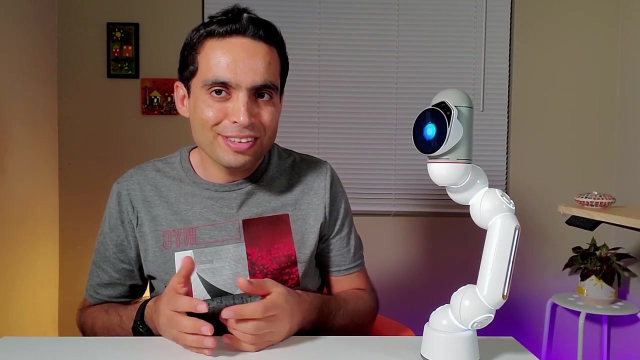 But fortunately Python's syntax is concise and easy to learn. Coding in Python is similar to the way humans speak, which makes it ideal for kids. Hey ClickBot, do you understand Python? Yes, I do. I'm bilingual. I can speak and communicate in both Blocky and Python. 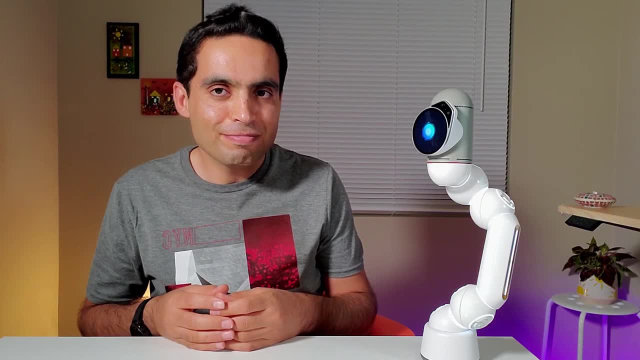 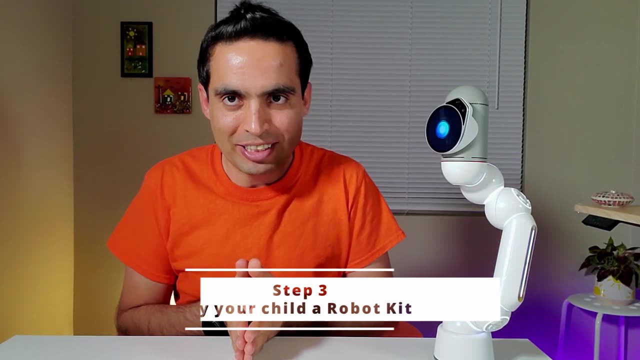 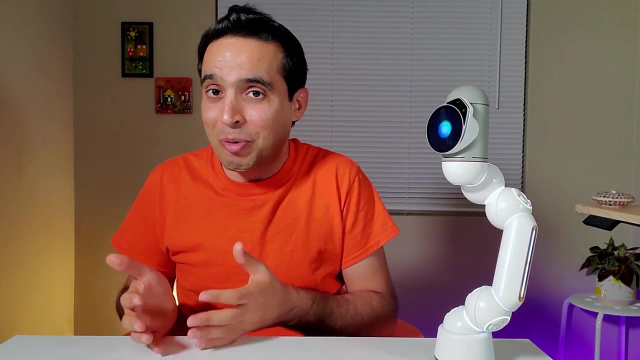 That's probably one of the reasons why I was selected as the best coding robot for kids by Forbes. Step number three: buy your child a robot kit. But why a robot kit? Well, kids are not like us, who can sit through hours of boring classes to learn a subject. 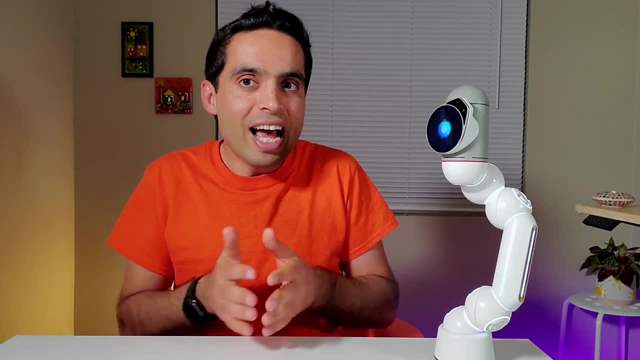 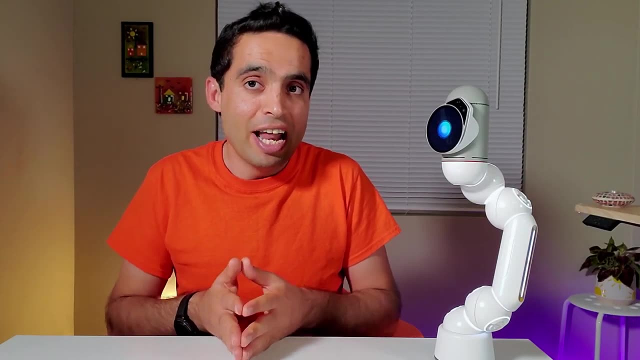 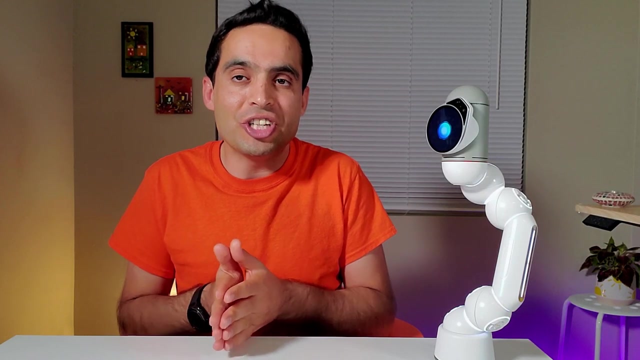 For kids, it's either fun or they're out, And that's why a simple but fun robot kit is the best tool to introduce your kids to robotics. Now the question is: which robot kit should you buy for your child? If you're looking for a robot kit that checks all the boxes I mentioned in this video, then ClickBot is your best bet. 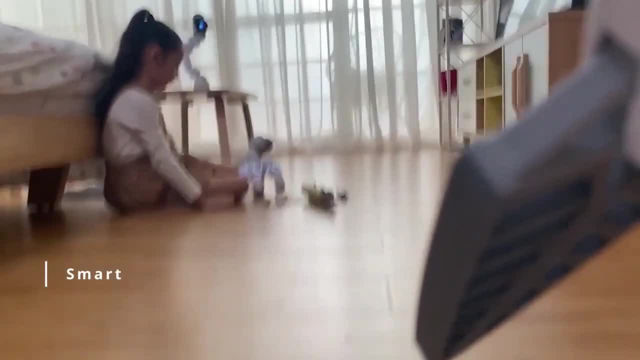 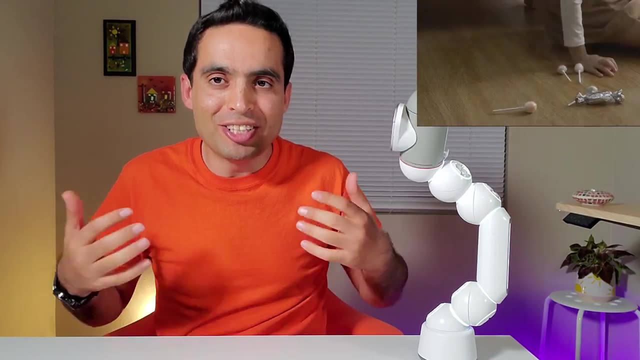 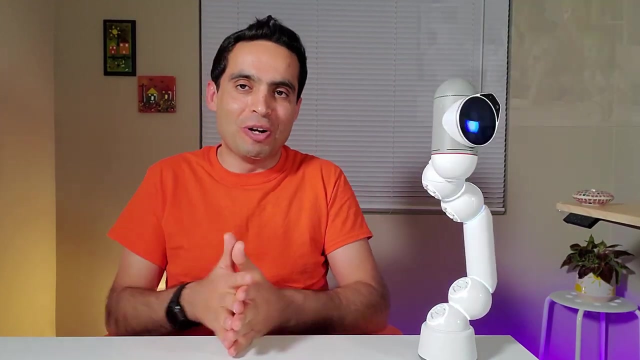 But why? ClickBot is a smart toy that is engaging and so fun to play with. Your kid will fall in love with it. I'm a robotics engineer and I design robots for a living. I've built and seen many different robots, And yet I have so much fun playing with ClickBot. 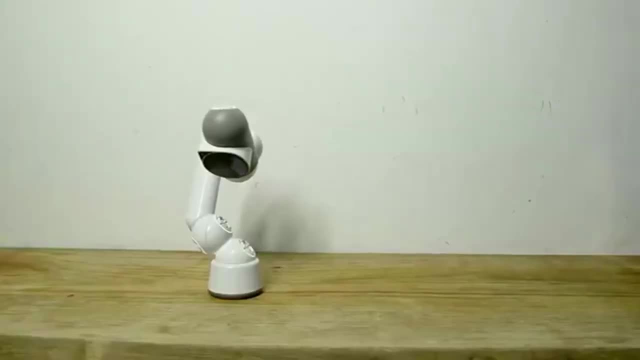 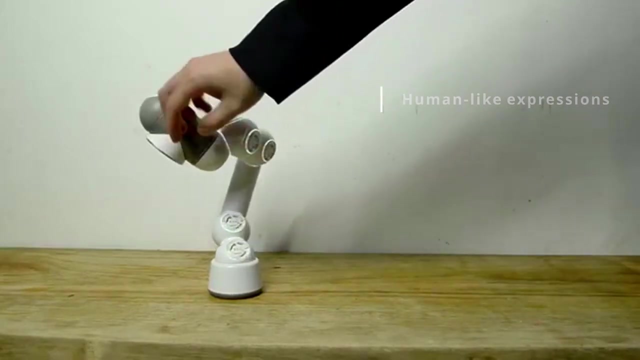 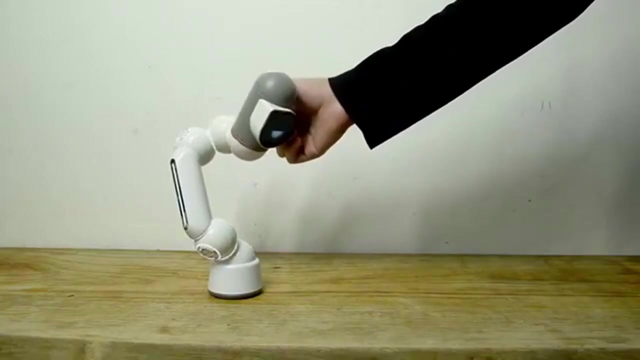 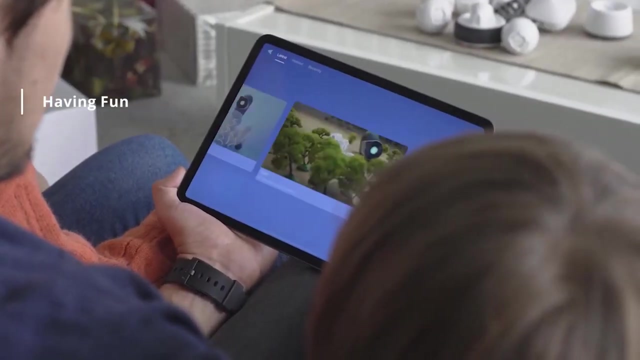 Well, being designed by a Pixar actor, ClickBot has so many human-like expressions that makes it feel like it's your personal robot, straight from a Pixar movie. With ClickBot, your kid will have a long-lasting fun and interest and just playing with it. chances are your kid will want to program it. 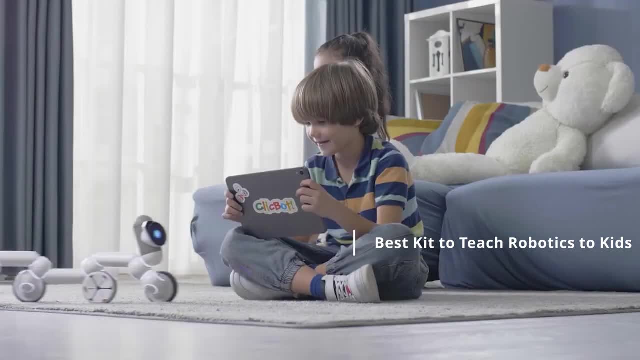 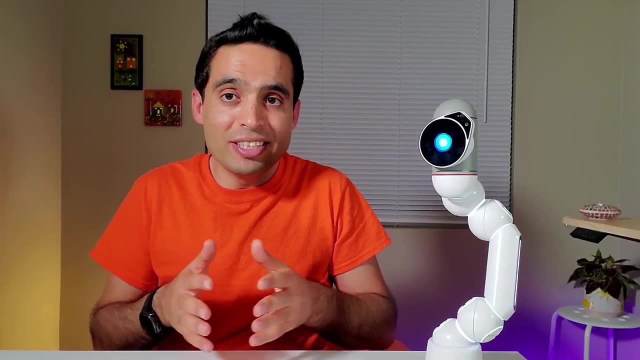 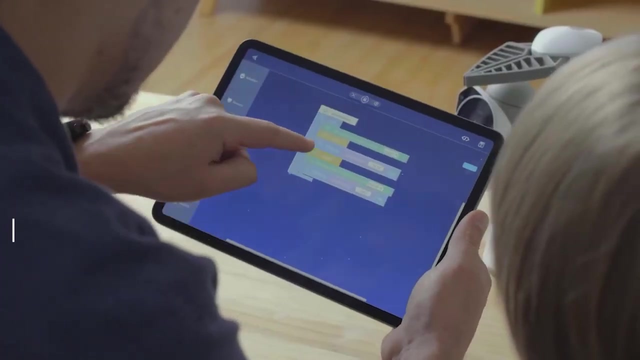 And just like that, he or she will love it And just like that, he or she will be introduced to the beautiful world of coding and robotics. ClickBot is the answer to how to teach programming to kids in a fun way. Younger kids can program it using Blocky and older kids can program it using Python, which is a language widely used in robotics.